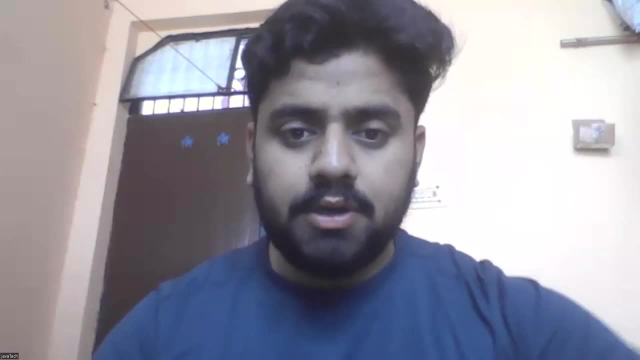 So hello students, hope you all are doing well. So welcome back And from today we will start the series of our JavaScript programming language. Okay, So either either you are you guys, know the some little basics concept of your any any programming language, or you are beginner in programming language. 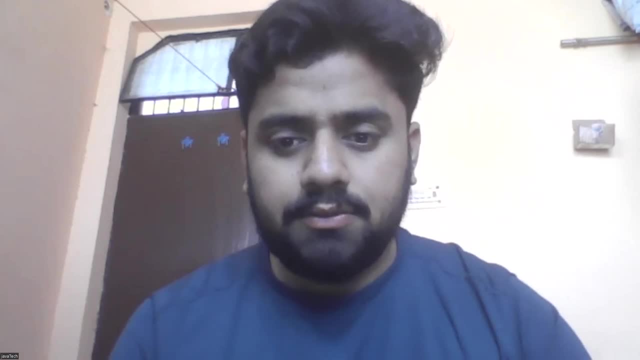 In the field of the computer science. Okay, So this all the playlist of your JavaScript is for you guys. Okay, We will. we will try to cover the each and every concept of your JavaScript programming language, from the basics to the advanced level. Okay, So just just follow our. follow the all the videos from from: 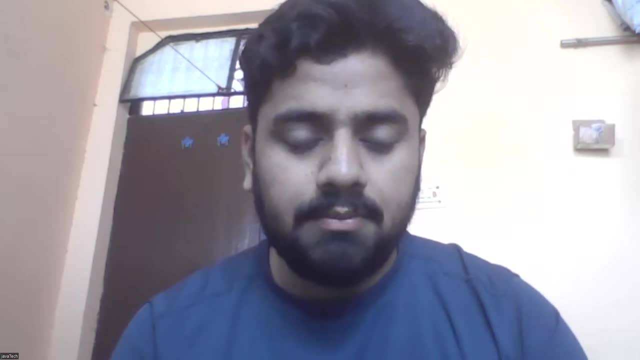 just beginning to the end, Okay, And I will make sure that if you follow the all the concept, or that I will, I will deliver on my channel then. then you will become definitely the proficient in JavaScript. Okay, So let's do not waste time and let's discuss about the JavaScript programming language. 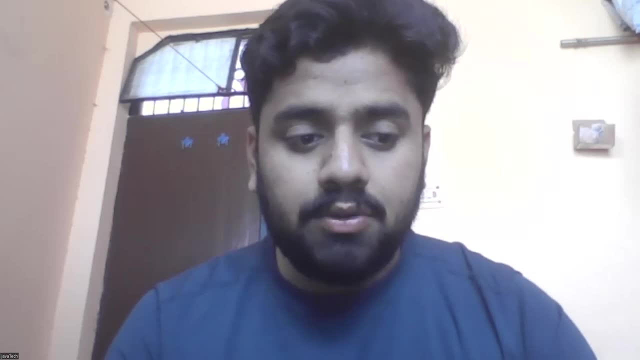 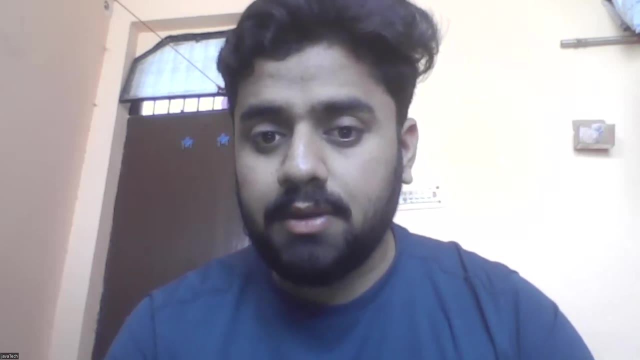 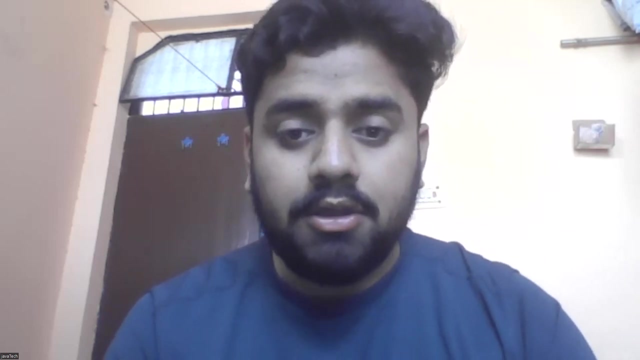 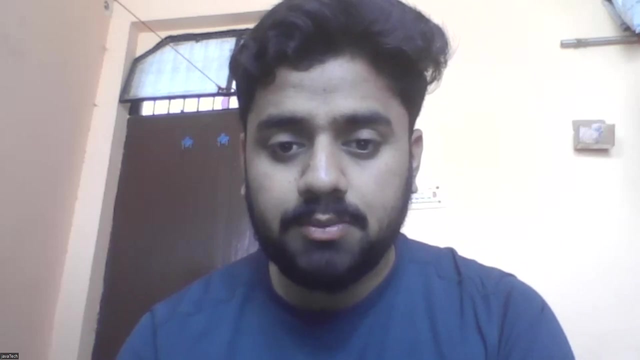 So that is what is JavaScript? Okay, So the basically your Java script or kind of your programming language, just like Java and Python are the programming language, Your Java, your Java script, is also a kind of programming language that is used for, that is used for interact with your operating system. Okay, And we had, we had discussed about that. 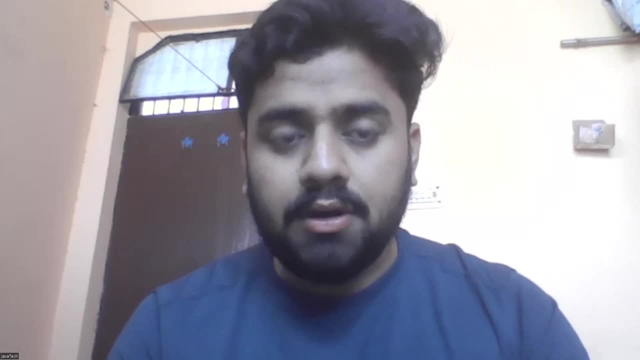 Your Java programming language, Okay. So if you wanted to learn about your Java, Okay, then I will. I will provide the link of the you know the Java playlist in the description box, or you can access our Java playlist as well from there. Okay, So, and basically, your JavaScript is also a kind of you know the programming language. Okay, And it is, it is. 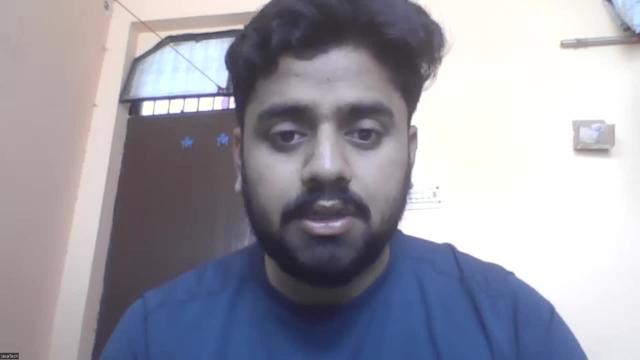 is mainly used. it is mainly uh used in the developing of your web applications. okay, see, java is mainly uh used for the developing of your backend part of your any uh web application. either it is a web application or either it is an android applications. okay, but the java script. 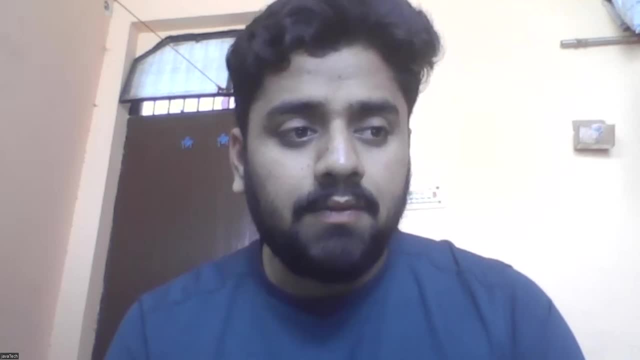 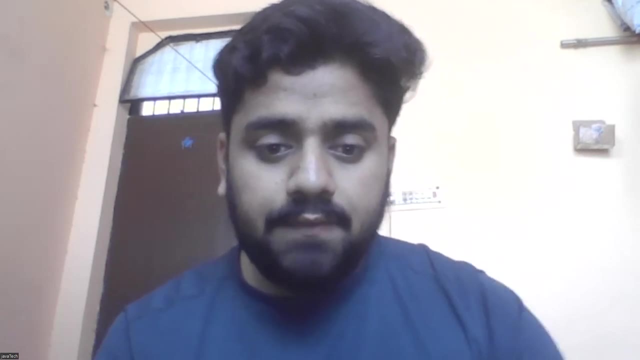 is mainly used for the developing the wave web application, or mostly the fronted part of your web application. okay, so, if, if i will, i will try to make sure you. uh, by using the real life example. that is, what is the main role of your java script in developing the web application. then 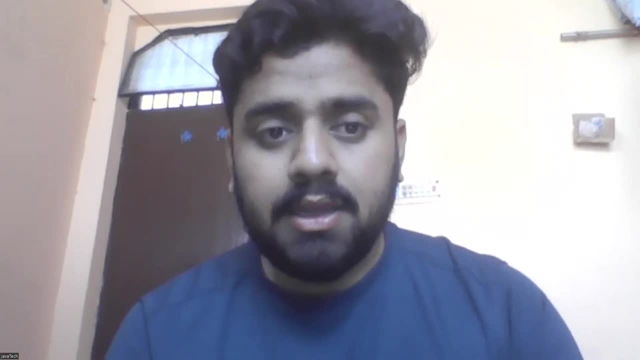 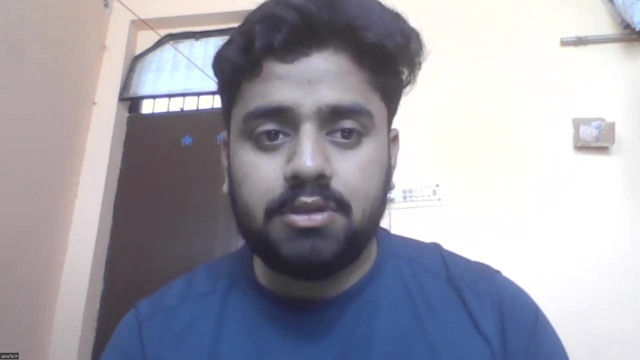 uh, let me share my desktop screen, then i can, i can, uh, i can give a real life example of your. uh, i know the javascript, that, how the javascript play a vital role for the developing your wave application, basically the front end of your wave application. okay, so see. 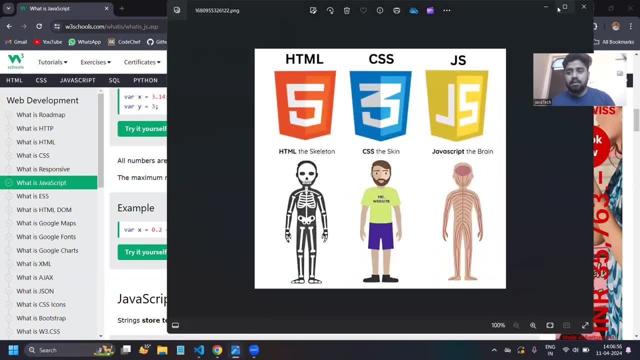 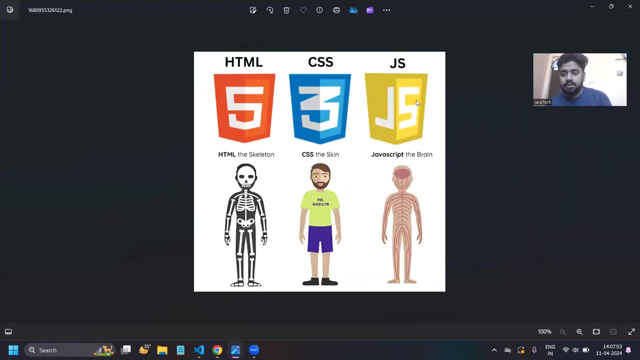 if, if i will take a real life, real life example of your javascript. okay, see uh for the for the uh developing any wave application, for uh developing any, any wave application, uh, basically the front end part, you have to uh require the three components, that is, html, css and javascript. 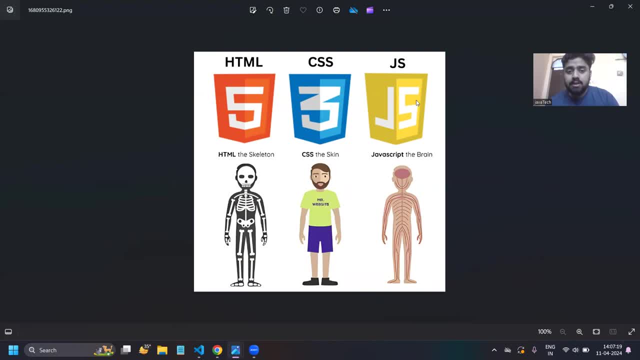 okay, the uh. basically, your html is. it stands for hypertext markup language. okay, and css is. css stands for cascade style sheet and the javascript, uh, javascript is a kind of uh, you know the programming language. okay, so i will. i will. uh, i know the. i will assume that if, uh, you are came for the learning javascript, then you guys are uh. 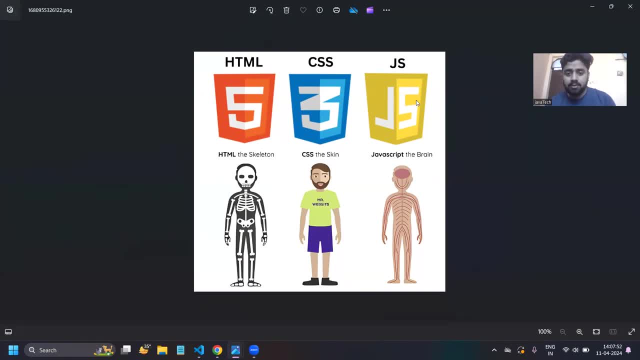 well aware about the html and css. okay, but if you want, then comment. okay, then uh, comment me, i will uh that. uh, you want the separate uh playlist on the html and uh css, then i will, uh, i will go for it as well, okay, but uh, this is the. 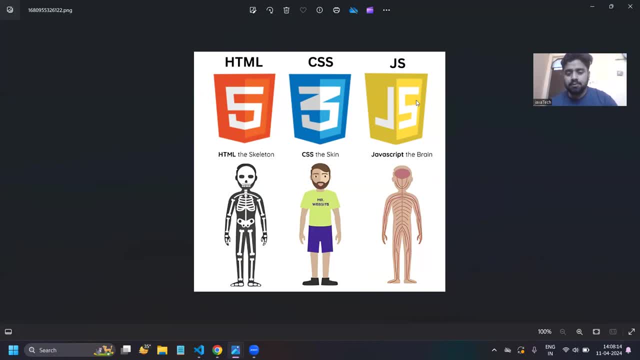 video of your uh basically, core javascript, okay, so, uh, we will not gonna uh not gonna deeply discussed about your html and css, okay, but if you want, then just uh drop a comment. i will uh make sure that i will uh gonna make a playlist on html and css as well, okay, so, if, if i will uh give you the brief, brief description about the. 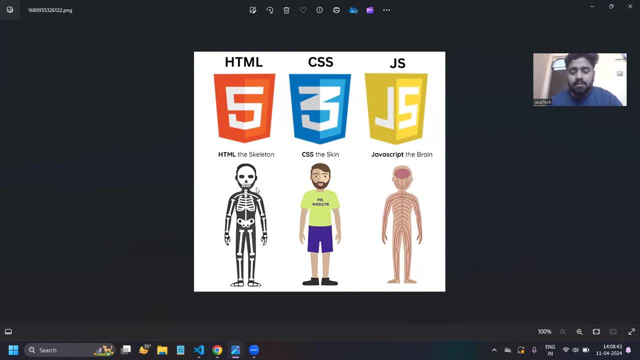 html and css. okay, see the uh. basically, uh, let's take a real life example. okay, your human body is a kind of a skeleton. okay, so only the skeleton. only the skeleton is defined by your html. okay, uh, means this structure of your body, the structure of your body is beingdefined by the html, okay, 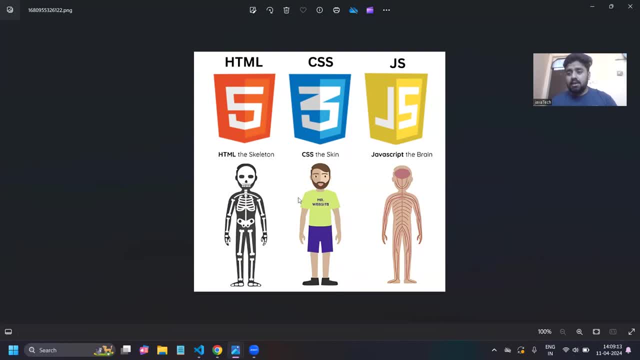 and then, after the skin, is skin, skin and the the color of your skin, the shirt, the band, the head, the bears, these all are defined by this CSS. okay, uh, basically, your css is used for the styling purpose and your html is used for, uh, the renders or your guide. what happens first is you are left, um bMac. 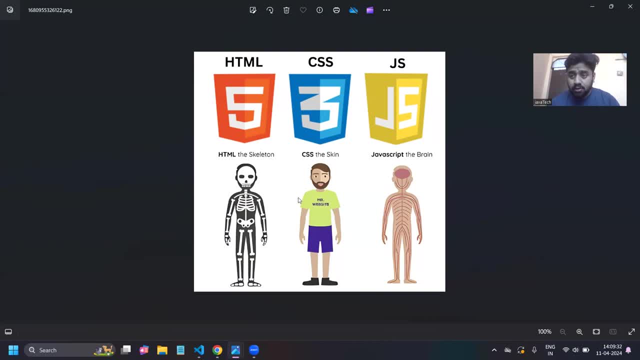 uh, we are, you are two guys bcc and uh, what happens first is you are bcc and you just giving the structure of your website, or obviously the front end part, okay, so your a structure is given by your, a skeleton in your body, and that is by your css. okay, and the style, the color, the looks, 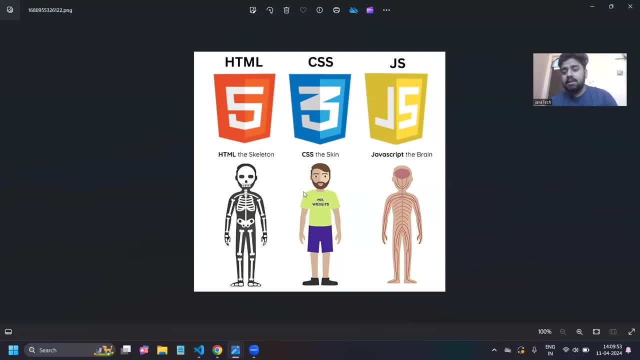 are given by your css, okay, and then see, the human body is uh here, prepared as well, okay, but but this person don't know that, how to perform any, any kind of activities. okay, this, see the person is being created here, but the person, uh, person don't have the thinking ability and uh, he can't. 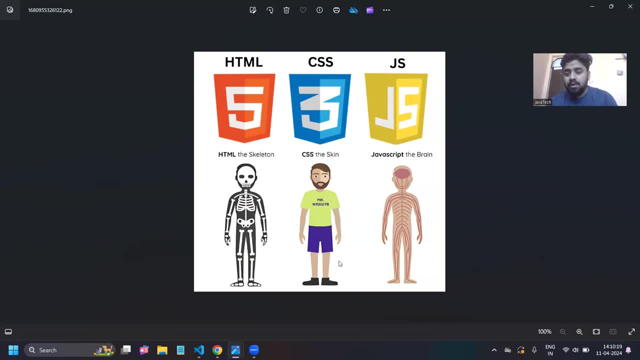 do any work. so if we have to make the person person automatic, we have to put a brain. we have to put a brain or any kind of functional automation thing that will make our personal automatic. okay, so if we put the brain, if we put the brain inside the 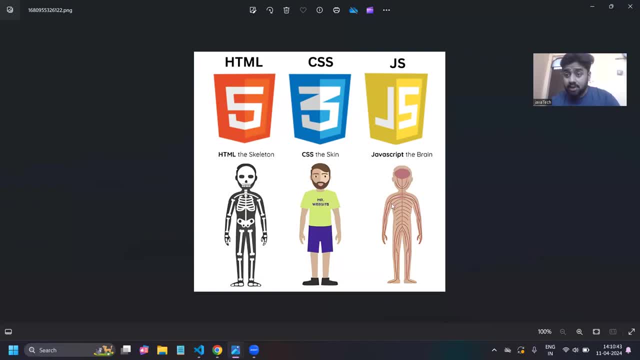 uh, human body, then that is the work of our javascript. okay, so our java, our javascript, will make sure that how your website will give response and how your website have to perform any work. okay, so the java script will make sure that how your website will perform any work. okay, so the java. 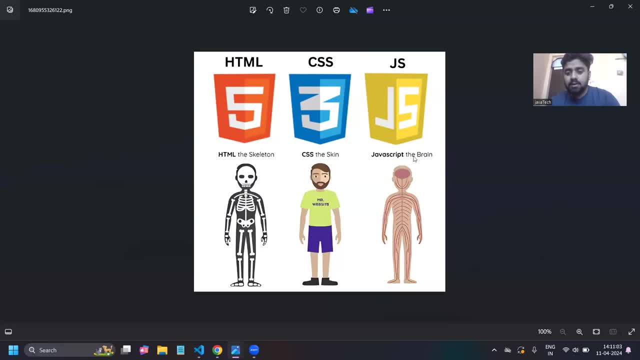 script will make your human body functional. okay. so, uh, if if i will uh briefly briefly define this all process, then the structure of your uh website is being defined by the html, then the styling part is being tip is being defined by the css and how your, how your website will work. 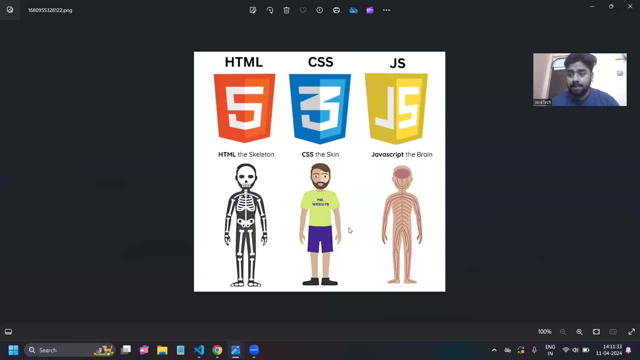 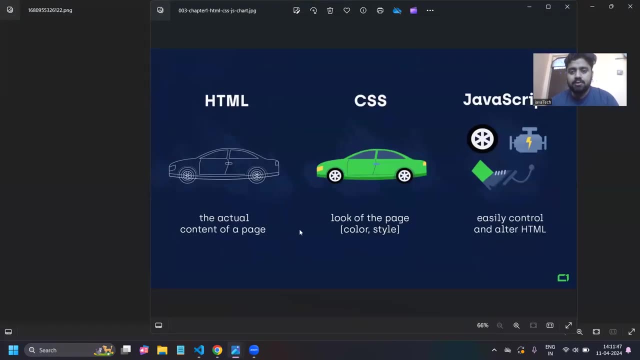 that is, that is defined by the javascript. okay, so, uh, your javascript will play the role of making your website dynamic and responsive. okay, and if i will take the another example, so okay, so, uh, here, this is your car. okay, this is your car here. i had make only the basic structure of my car, okay, i had. 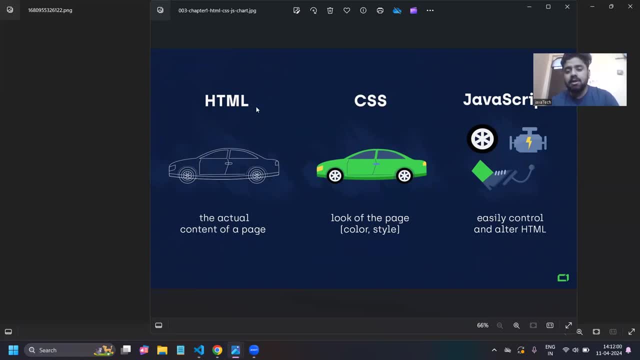 make only the basic structure of my car by using my steam, well, okay. and then after, uh, by using my csv, i had put the colors design on my car. uh, okay, of colors design styles on my car. and then after, see, my car is being red here, but 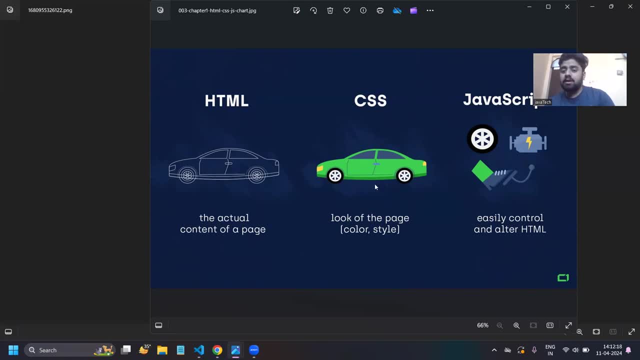 it doesn't contain any kind of angels. okay, that, uh, that see, the car is being made. okay, but it uh doesn't uh have the uh features of uh running, driving or anything. okay, but those feature can be installed by using your javascript. okay, so the engine part is being 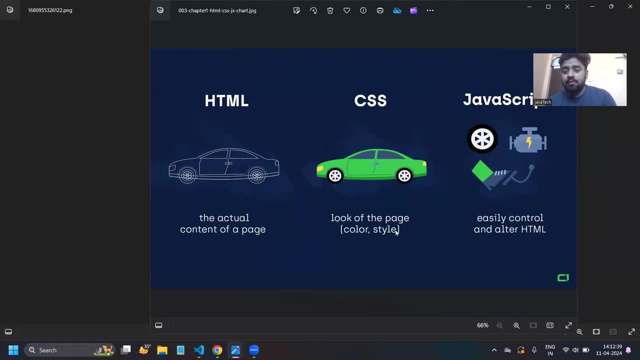 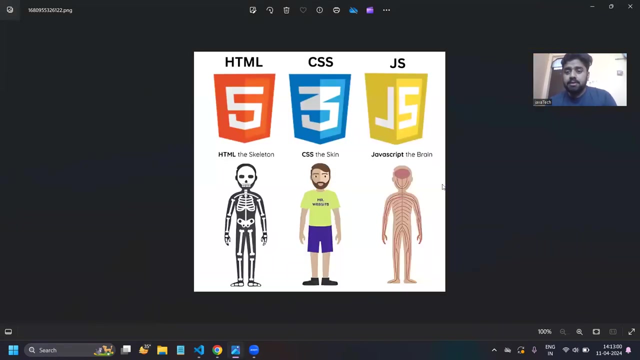 defined by the javascript. okay, that is how your car will gonna make functional, is this? all thing will be defined by your javascript. okay, so this is the basics concept behind your javascript, behind using the concept of javascript in the development of your web applications. okay, so this is the basic, basic, introductory part of your javascript, and in our next lecture we will